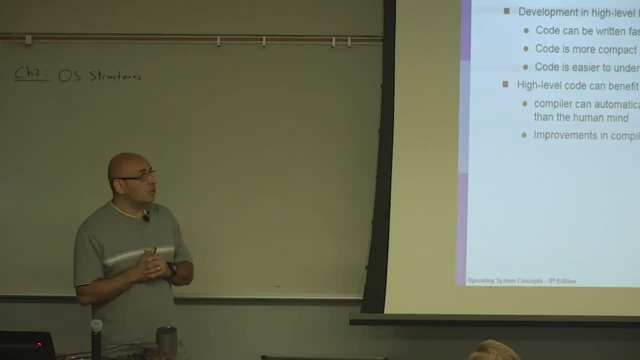 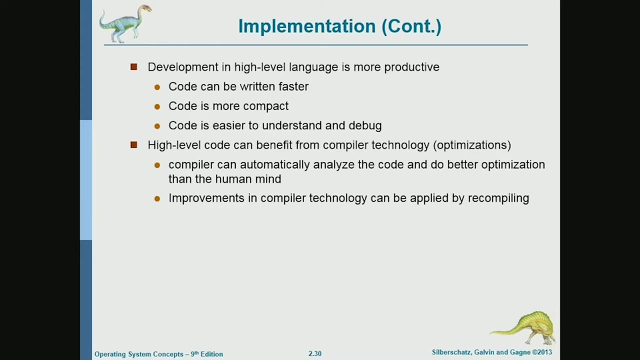 in a high level language as opposed to assembly. And these advantages are software engineering advantages. so more programmer productivity, easier to write, easier to debug- all the reasons that make people develop programming languages, human-like programming languages. In addition to that, there is a portability reason. There is a portability advantage because 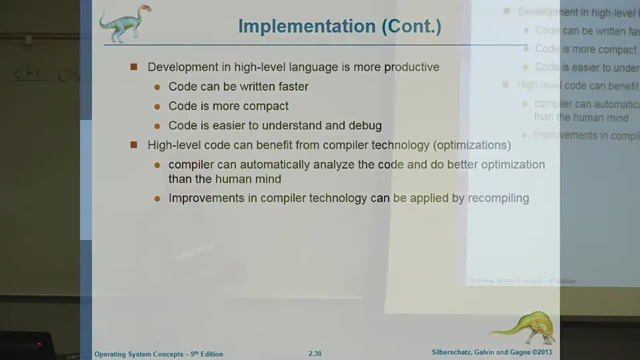 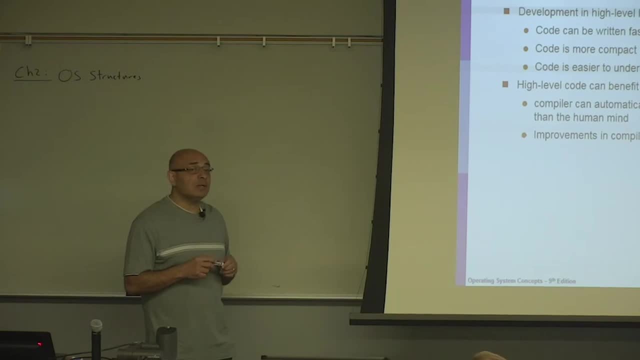 if you write in a high level language, you can port it to different systems. You can run the same OS on different systems. And what was the example that we mentioned last time for portability? Yeah, Yeah, Linux. And what are the different systems that Linux? We gave examples of three. 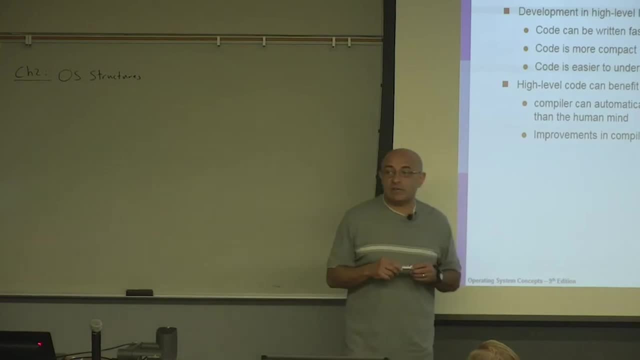 different architectures on which Java is run, Sorry, on which Linux is run. What are the three different systems? X86.. X86.. Intel X86 is one of them, PowerPC- Is it PowerPC? PowerPC and Spark. So at least three examples. totally different architectures on which the 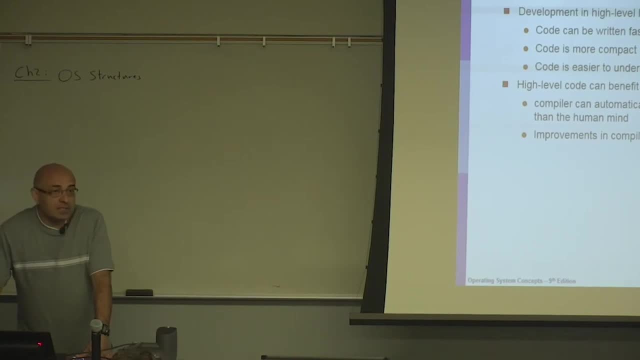 same operating system is run, And this is possible because the operating system is written in C, So we just compile it using different compilers. We compile it with a compiler that generates X86, and it will run on X86.. Compile it with a PowerPC compiler, and it will run on PowerPC. 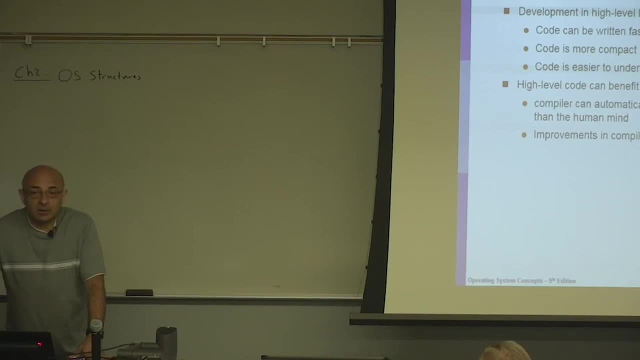 Okay. The third advantage is compiler optimizations. So when the operating system is run is written in a high level language, it will benefit from compiler optimizations And, generally speaking, the compiler produces does a better job than the compiler. It does a better job at optimizing code, at generating optimized code, But in certain 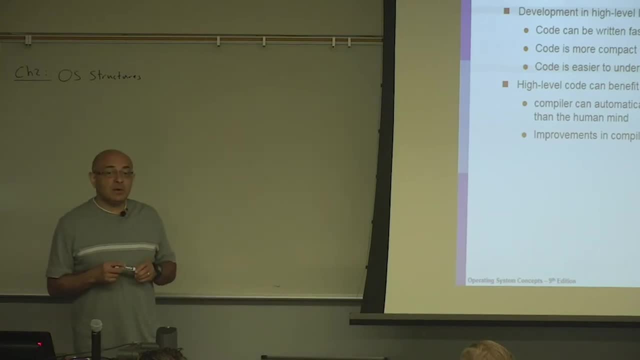 cases, writing code in assembly may make sense. When does writing code in assembly or specific pieces of code in assembly? when will that make sense? Yeah, Is performance critical? If it's performance critical, and so that's what we're going to do. 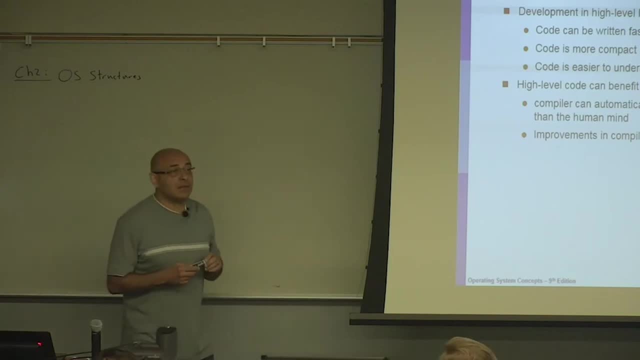 Okay, What's the other condition? It's small in size. Yeah, small, Yeah. So if you have a section that is performance critical and small, then an assembly programmer is likely to produce very efficient code for that particular section. So if it's not performance critical, you know why bother. If it's performance critical then you may consider writing it in assembly If it's small enough for an assembly programmer to optimize. But if it's a large piece of code then the compiler will be more likely to generate better code to optimize that. Because you know automation, the compiler is an automation, And automation always works better when you have bigger data to process. The kernel is written in a high-level language. Yeah, So most kernels, the kernels of the most of the systems that we use, are written in. 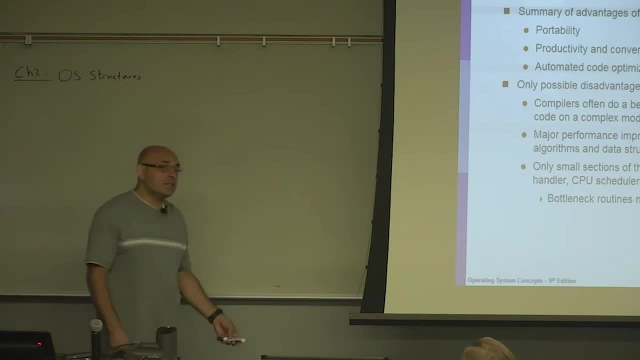 C. So we use Windows: the kernel is written in C. Linux: the kernel is written in C. Android, as we will see. you know, Android is based on Linux, so the kernel is written in C And the Mac OS- Apple's OS- is written in C. 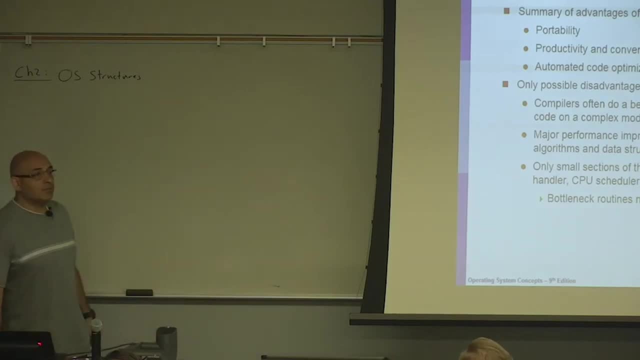 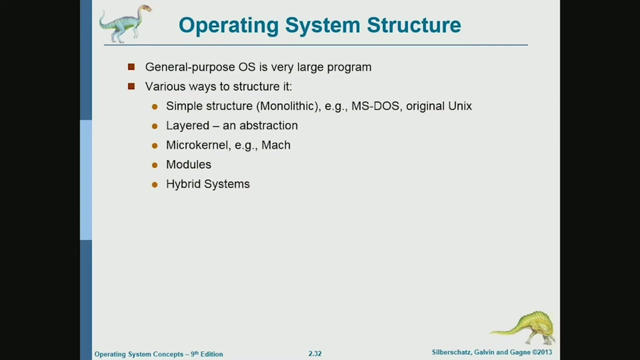 So very much all the operating systems that we use are written in C And that's why you know, in this course you know we must do some system programming in C. Okay, So now operating system structures. We will be discussing four kinds of structures. 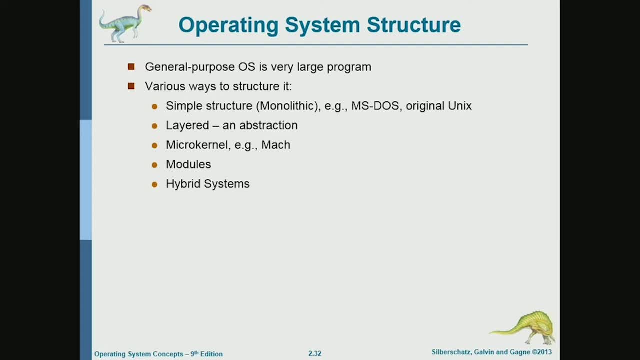 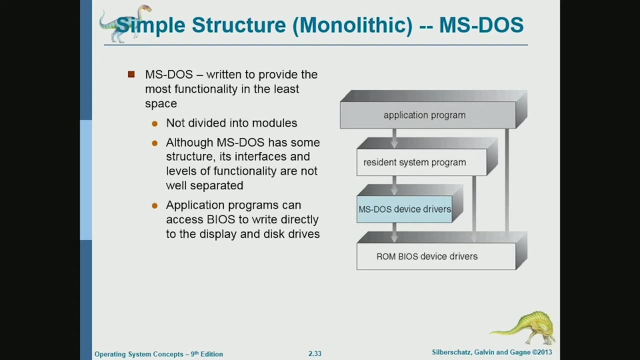 The simple monolithic structure or no structure, basically Layer, microkernel and modules. Well, let's see what each of these means. Monolithic, it just means that the operating system is in one piece and it's not divided into modules and it's not structured. 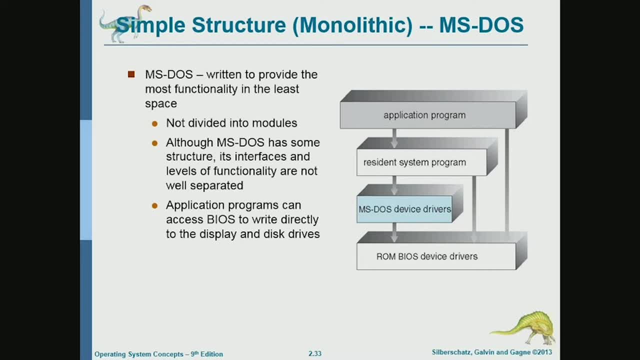 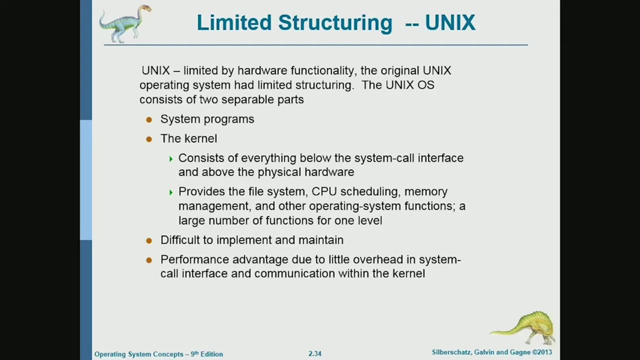 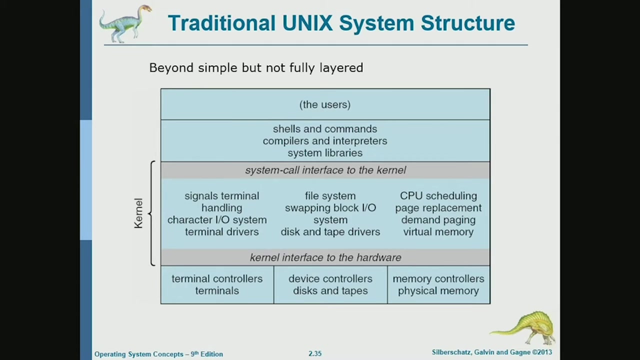 And one example is the DOS operating system, which was a relatively small operating system That offered limited features, And the earlier versions of Unix. So the earlier versions of Unix were to a great extent monolithic. By the way, as we will see later, real operating systems use a combination of approaches. 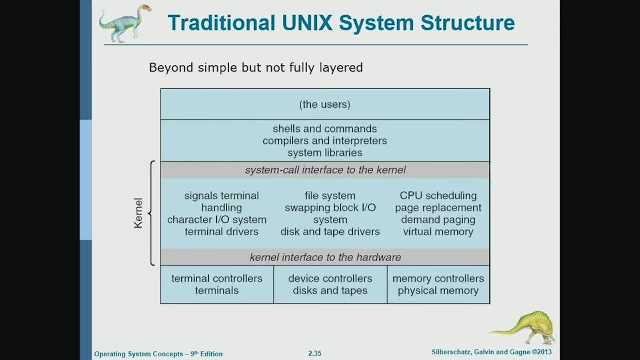 So, as we will see, all real operating systems are hybrid systems, So they use a combination of the approaches that we are, that we will be discussing here, So there will be no pure- there is no pure- operating system that uses a single approach. 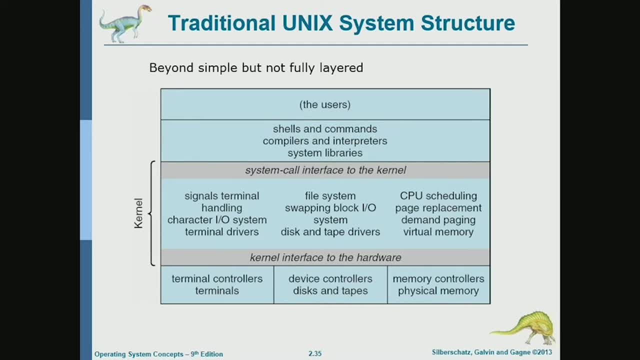 Why? Because operating systems evolve. It has to do with the way they evolve. You know, they start off by designing an operating system in a certain way. then they realize that they have a performance problem. So in order to fix that problem, 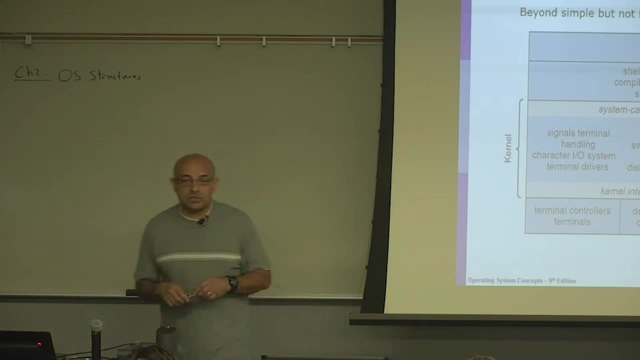 So, in order to fix that performance problem, they take a different approach And you know, sometimes an operating system is based on another operating system, like Android is based on Linux. So it's not a new operating system that was written from scratch. 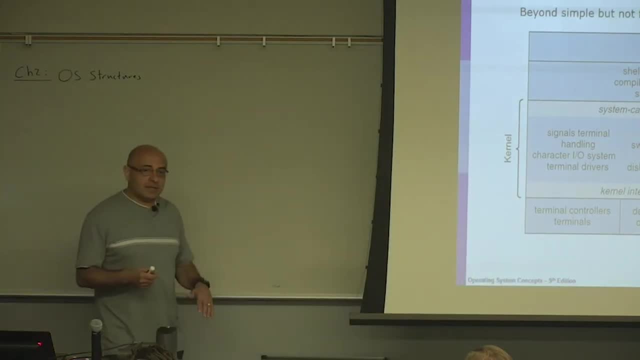 So you are building it on an existing operating system, but in the components that you are adding you may take a different approach. So the way operating systems were developed, in reality they made them all hybrid, you know, mixed using a mix of approaches. 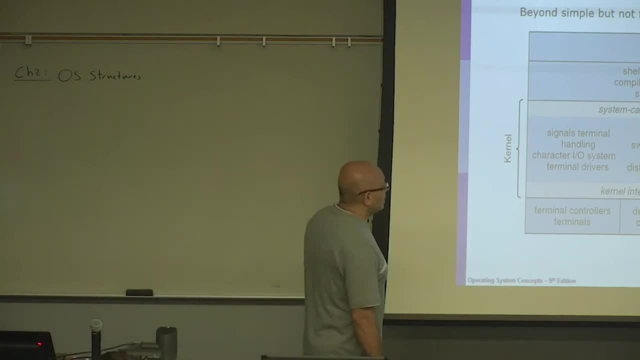 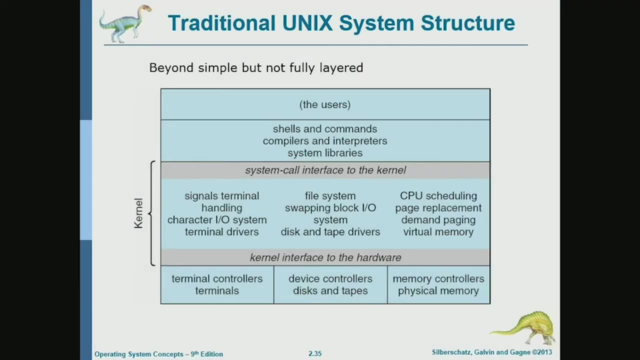 So if we look at a classical Unix system, we will see that there isn't much structure. We have a big kernel that has very much everything in it And there is an interface to the hardware and an interface to the user, But between these there are all the services that the kernel provides. 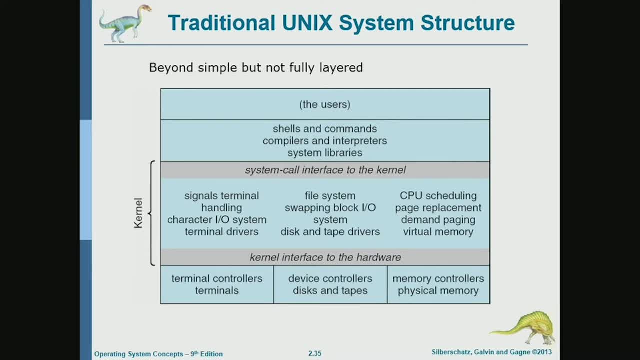 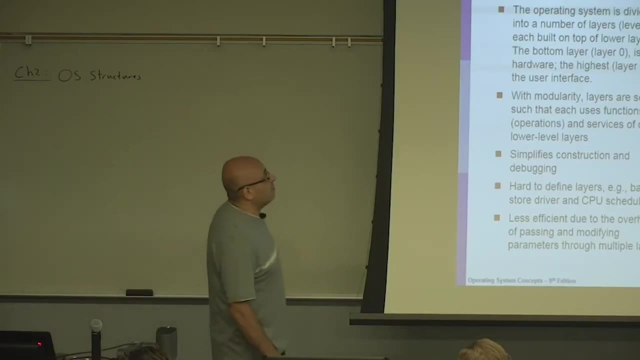 So this is monolithic, In the sense that there is a big kernel that has everything and it's not well structured. Now we will understand what this means when we look at the other approaches that are more structured, And the first approach that we will look at is the layered approach. 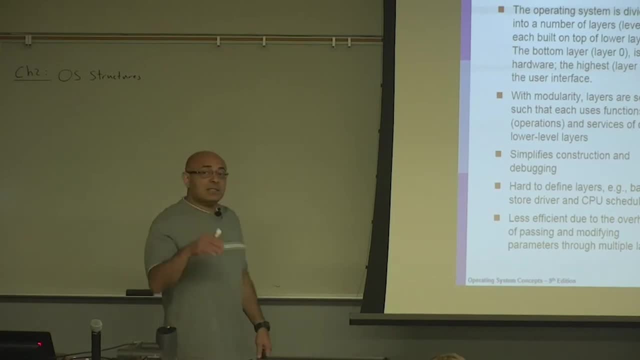 In the layered approach, the kernel is organized in layers, So there is a hierarchy of layers And there is layer zero, which is the hardware. On top of that there is layer one, So this is the lowest level layer in the system. 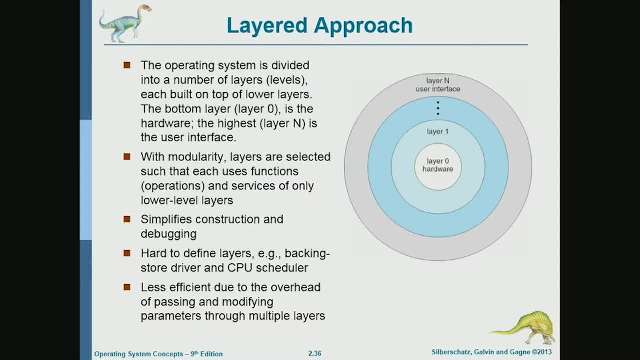 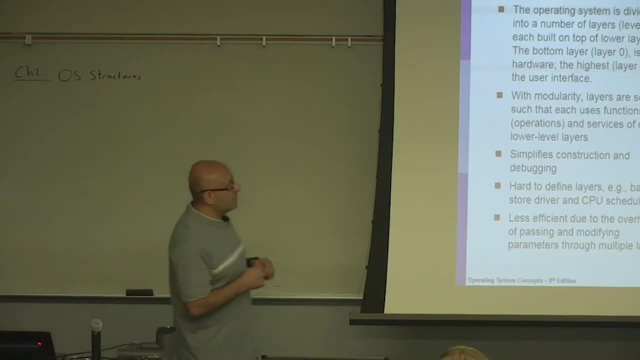 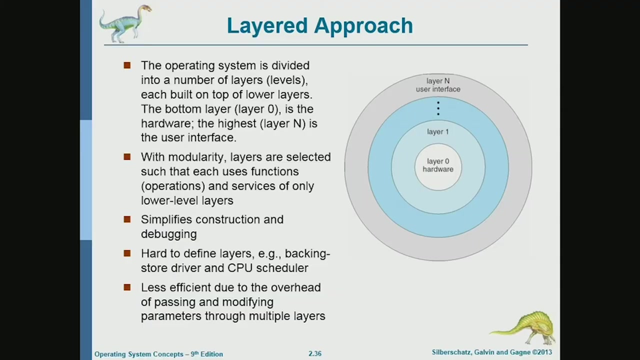 And this kind of approach is an abstraction Or it's an ideal approach that probably no real operating system implements exactly. So you may see this kind of approach in some operating systems, But it's not going to be that the whole system is designed using this way. 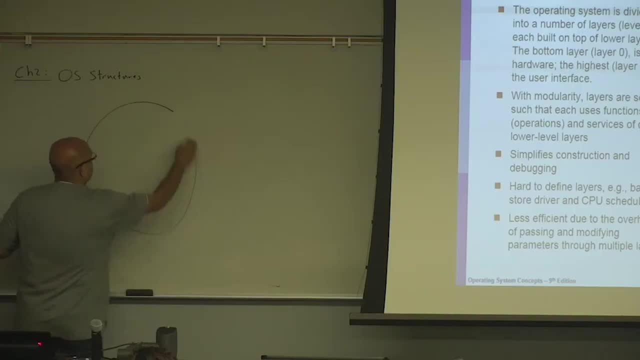 This is a hierarchical, So if you have multiple layers and if you are in this layer, there is a service in layer n, then this service can only call services in layer n minus one, So it cannot talk to the layers above it. 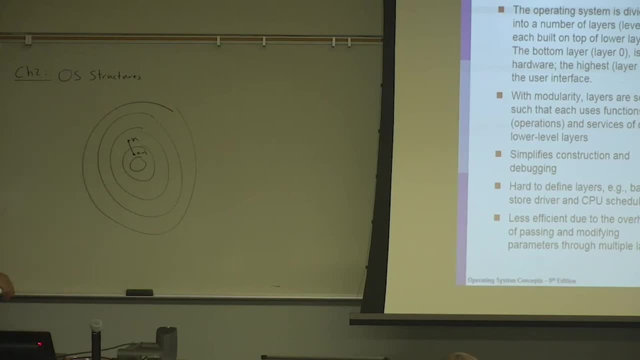 And it cannot even talk to the layers that are below it but are not next to it. The only layer that this can talk to is layer n minus one. So you are at this layer. You're basically calling, making function calls that are in layer n minus one. 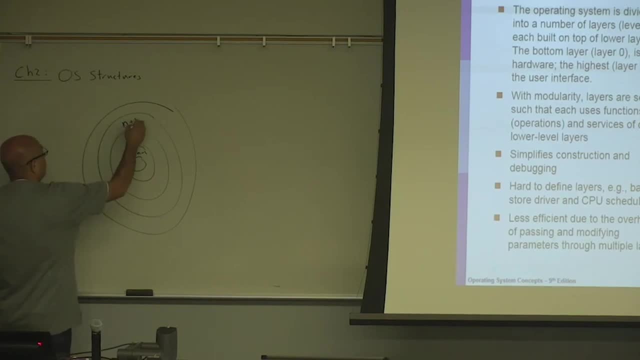 So if you are here n plus one and you need to talk to n minus one, you have to go through n. You have to go through the hierarchy, Okay, So. So the question is: what are the advantages and disadvantages of this approach relative to the monolithic? 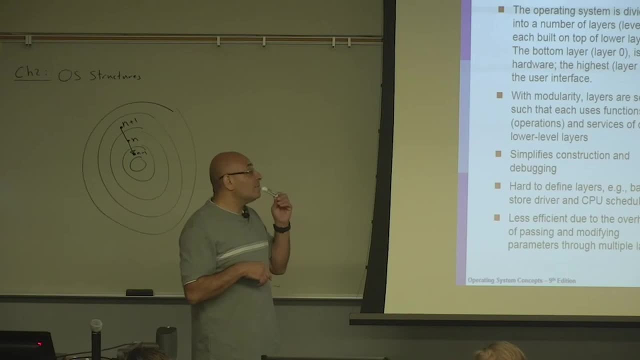 Yeah, Performance. So which one has better performance? layered or monolithic? I guess it would be monolith. I guess it would be monolith. Yeah, Monolithic. Why Well, the layers. If one layer needs to talk to a layer that's much below it, it has to go through open. 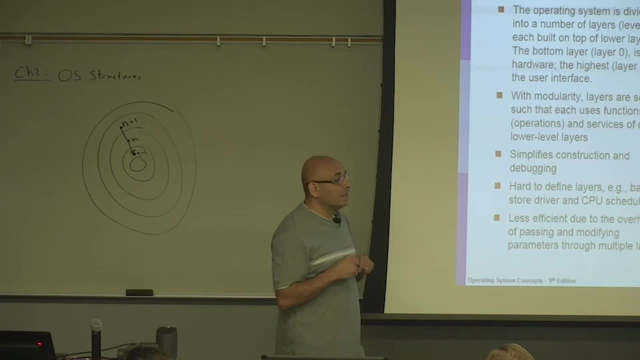 a bunch of other layers which takes up more time. Yeah, exactly, So that's an overhead. You know, going through that hierarchy or having to go through the hierarchy will involve an overhead which will degrade performance. So from performance point of view, monolithic works better than layered. 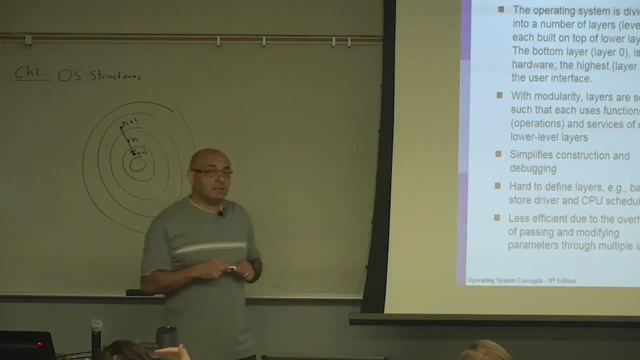 Is it more simple So you don't have to worry about what's coming in one layer and what's going out one layer. You don't have to worry about this whole net of communication that might be happening. Okay, So here you know. the word simple is not very so it could be interpreted both ways. 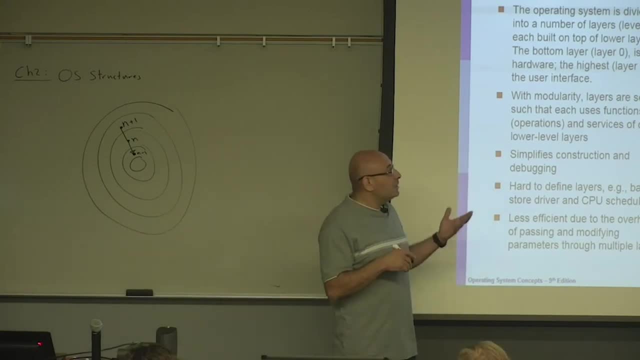 I mean simple. you can argue that this is simpler, but you can also argue that monolithic is simpler because there is no structure. In fact, when you say simple monolithic is simpler because it has no structure, This is not simpler, but it's easier for development. 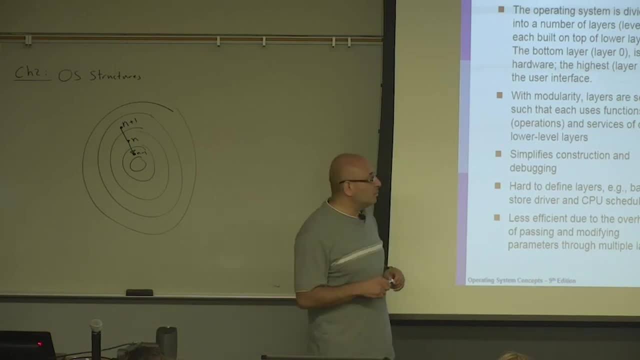 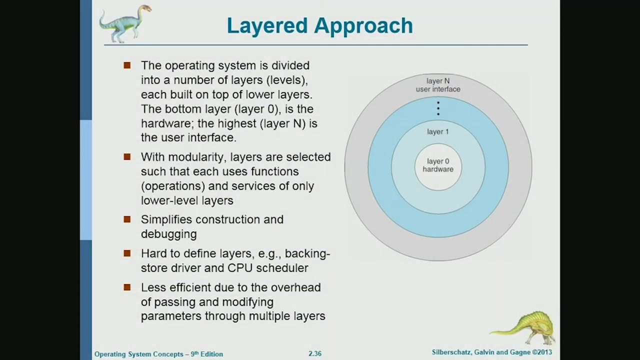 Development and debugging. and when you are debugging this, when you have multiple layers, you can debug each layer separately. So, basically, this is the you know, this approach has the good, all the good ideas that you learn in software engineering. 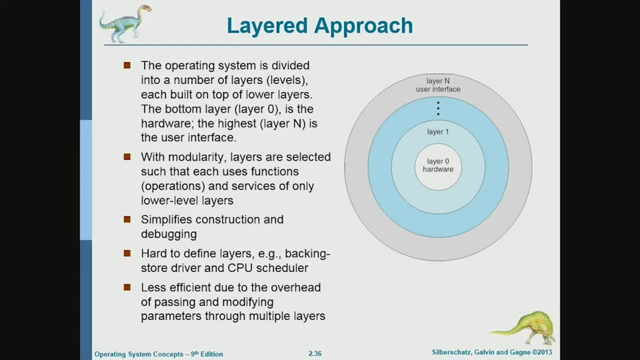 So, from software engineering point of view, this is a top-down design, Okay And it has all the advantages, all the good things that you learn in software engineering classes, While a monolithic kernel, from software engineering point of view, is terrible. 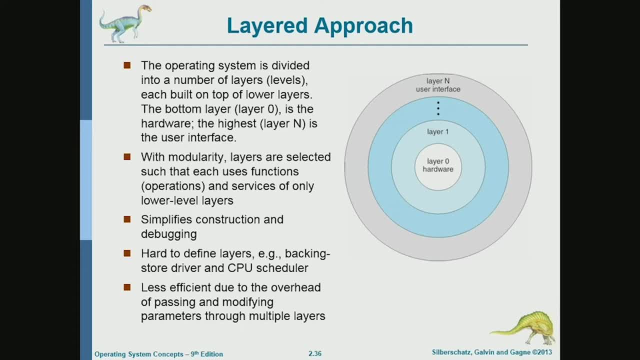 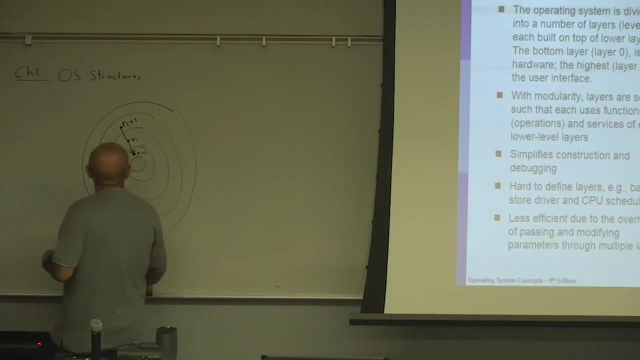 Right, It's not modular, It's not divided into pieces, But from performance point of view it's good because there is minimal overhead. So basically, this is, you know, cleaner design, Better from software engineering point of view, But from performance point of view, monolithic is what's better. 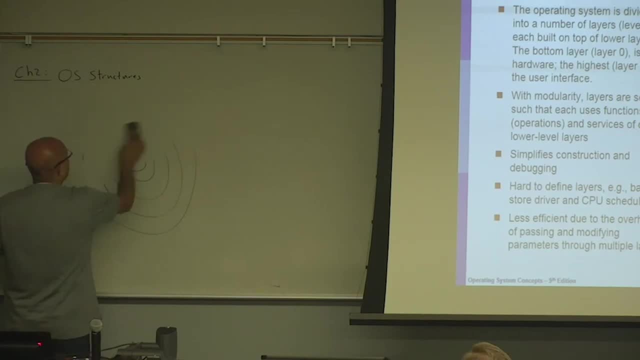 Now one disadvantage or one, I wouldn't call it a disadvantage, but I would call it an issue or a challenge. a challenge in designing a layer system is that sometimes it's not clear where to put a certain service, or given two services, X and Y- sometimes it's not clear. 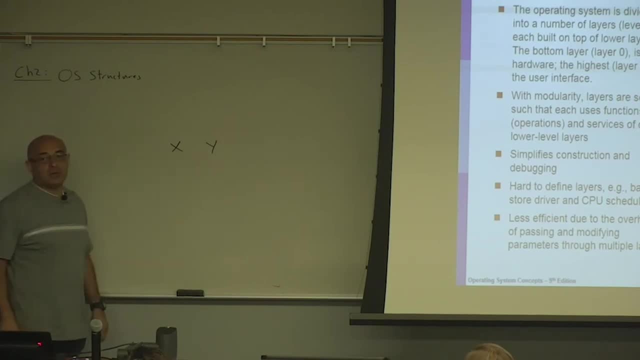 whether X should be on top of Y or Y should be on top of X. So in order to understand this, we need a concrete example, And the concrete example is the CPU scheduler and the back store, or the disk driver, Disk manager, Disk manager. 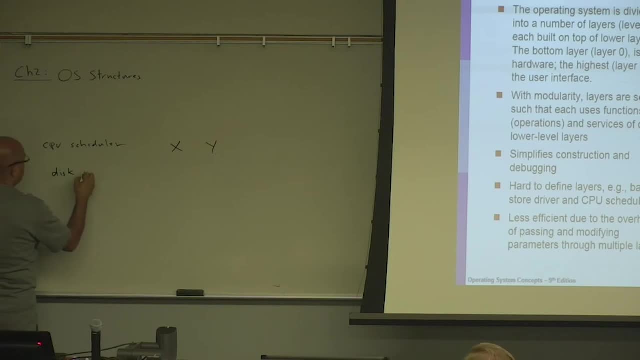 Or what they call the back in store driver. So on the surface- well, on the surface it's- the disk driver appears to be on top of the scheduler And the disk driver uses the scheduler. So the scheduler is at a lower level because the scheduler schedules all processes in the 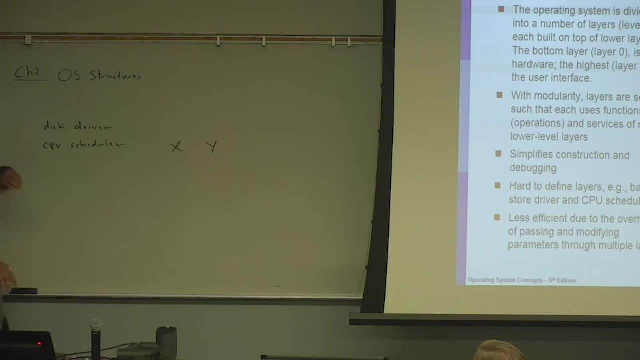 system including the disk driver or the disk manager. So the disk driver needs or uses the scheduler And the scheduler is at a lower level. This is what it, what appears on the surface. but if you think deeply about this and the needs of the scheduler, the scheduler may need the disk driver if there are too many. 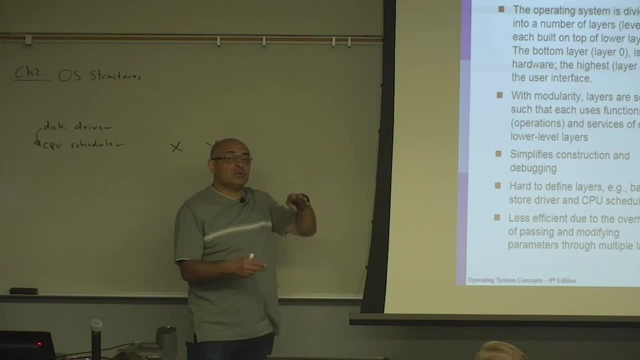 processes in memory and the scheduler needs to swap some of them to the disk. So if it needs to put some of the processes on the disk because there isn't enough memory, in this case the CPU scheduler will be invoking the disk driver. So in this case, the, the interface, will be invoking the disk driver. 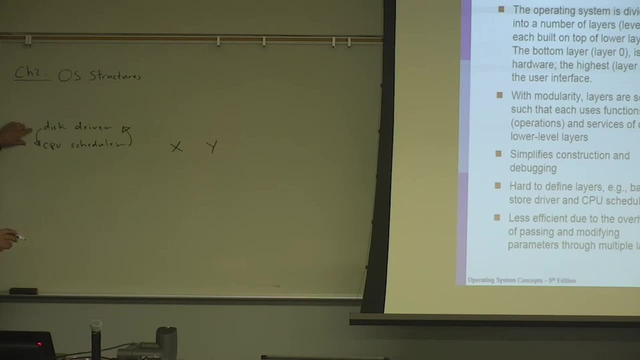 The. the interaction goes in both directions. When the interaction between two layers goes in both directions, it will not be easy to decide which one should be placed on top. Now. one solution is to just put them in the same layer, put them both at the same level. 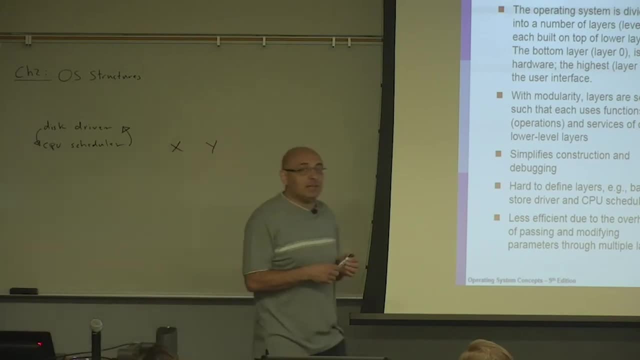 But if we keep doing this, what will we end up with? Mono? Yeah, It will end up being mono, It will end up putting everything at the same level. So this is just a challenge in designing a, a layered approach, And I think it's it's a challenge that we always face when we try to to do a top-down. 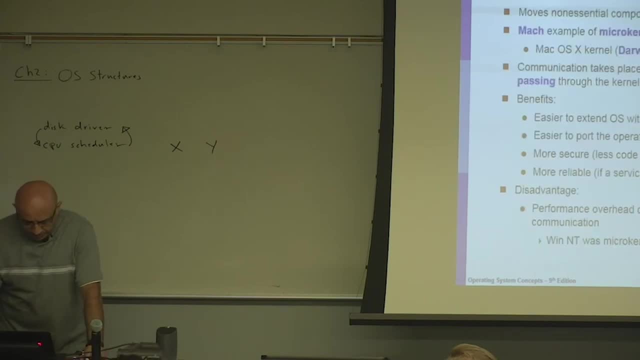 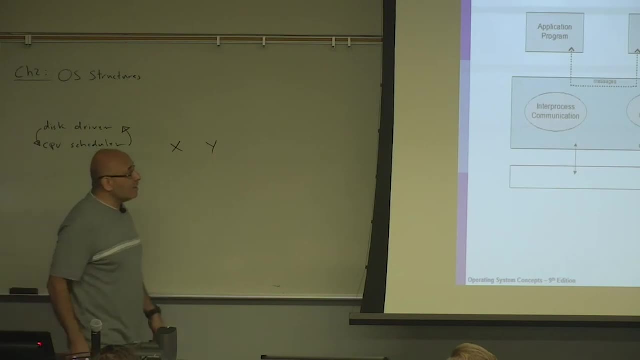 design. Okay, now the microkernel system. Now, with the microkernel system we have a small kernel That has only the essential features And all other services. all other services are placed in separate processes that are run in user mode. 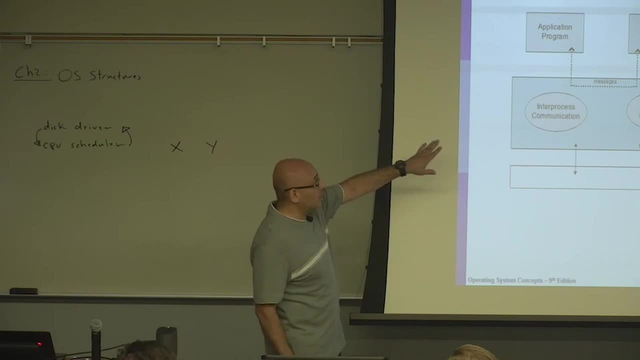 Now, this is just an example, So don't think that all microkernel systems are going to put these services in the kernel and these services outside the kernel. This is a design decision and different designers may make different decisions and may choose to put different services in in different places. 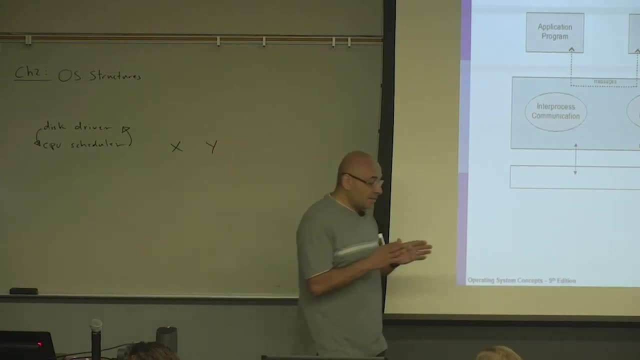 But the idea is, the designers of the system are going to identify what they think are the essential services And only those essential services are put in the kernel, While all other services are just run as separate, separate processes in user mode. Okay, So when? when these separate processes, these separate processes that are run in user mode. 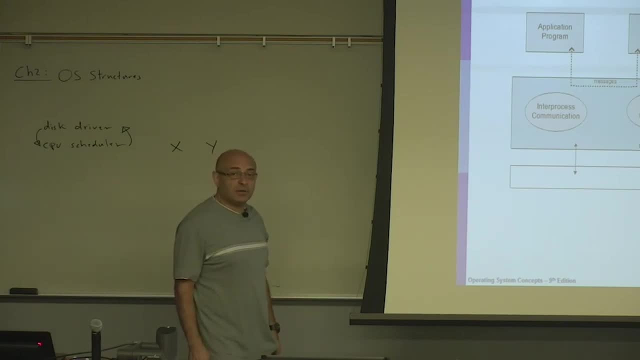 cannot talk to each other directly. They have to go through the kernel. So if you have an application program which is running in user mode, if it needs a- you know- a service from this, it needs to make a request to this service. it cannot talk. 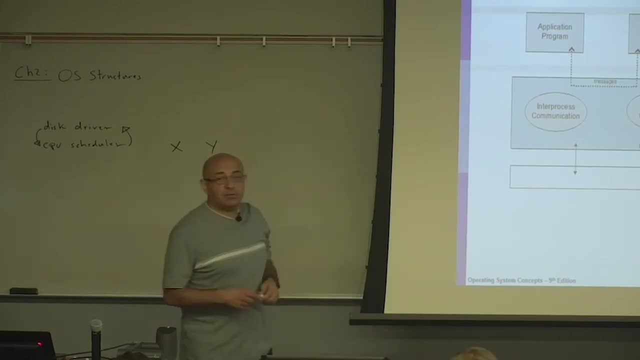 to it directly. It will communicate with the kernel Through messages And then the kernel will communicate with that service and the kernel will then return the result back to the application program, And this is done via message passing. Okay, So now the question is: from a performance point of view, is this good or bad? 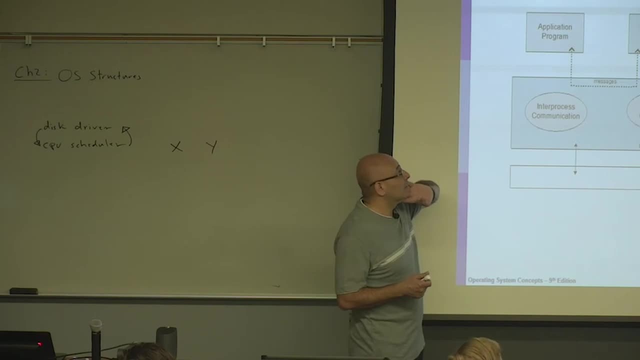 Bad, Bad, Bad, Bad, Bad, Bad. It's bad. So there is there is an obvious overhead in those messages that are exchanged between different processes. So there is the message passing overhead. Now this leads to the logical question. 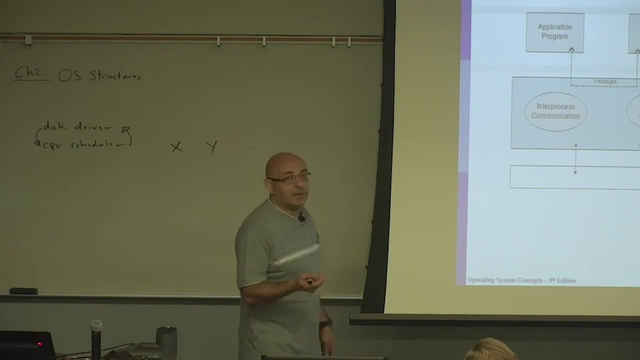 What's the, the next, you know logical question? I mean, there is an overhead, So what should we do? Questioning What's good comes from this system? Yeah, So what's? what are the advantages of this system and what made people come up with this? 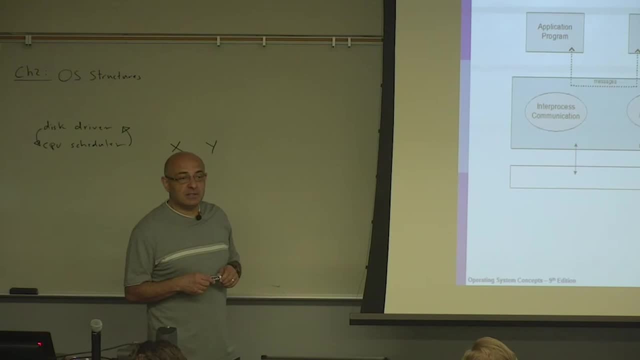 approach, It must have some advantages. So Looks like everything is easier to define. Maybe we don't run into those same issues that we did in the layered approach. Okay, Things are easier to design. Okay, We do not have the hierarchy. 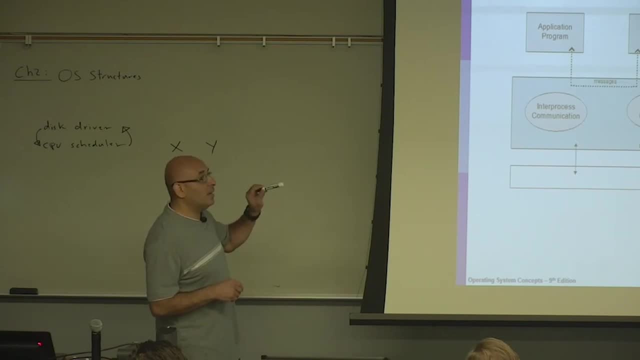 So here we do not have the hierarchy that we had in the layered approach, So any so. so different services can talk to each other without going through the hierarchy, but they have to go through the kernel. So this is: yeah, this is one advantage. 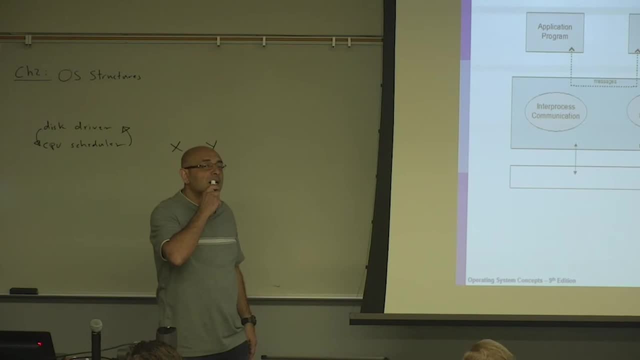 Yeah, All the user services can interface with the common, can use a common interface to the kernel. So it only you don't have to know all the other, all the other user services that you may want to talk to or how to interface with them. 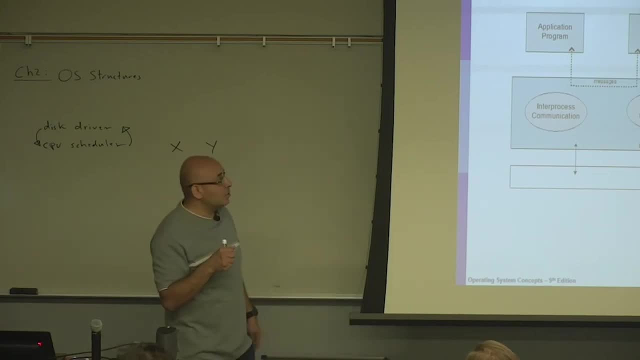 Yeah, No, but even in other approaches you, the user process always talks to the kernel, It's not. the user process will always talk to the kernel. It's not going to talk directly. Yeah, Much more security in this one. 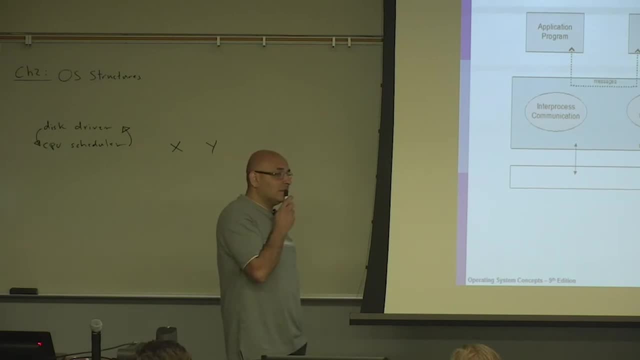 Why is it more secure? Because the application program, if it is trying to access some file of this system, it goes through the kernel and kernel can let them know like: is it secure or no? Does the user have the permission to go through the file system or no? 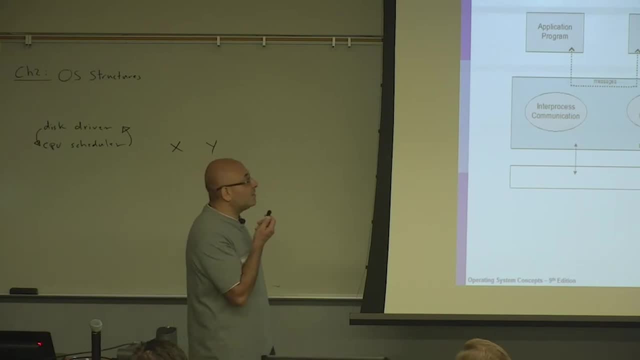 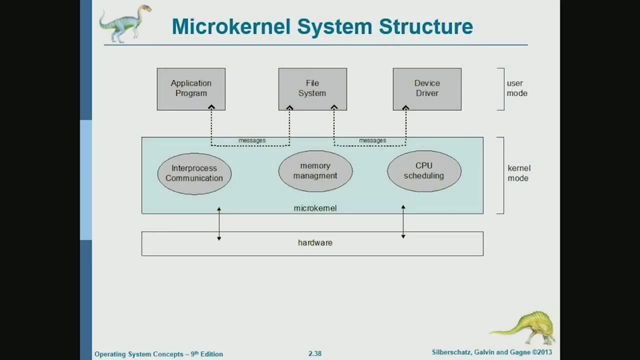 Okay, But we would have the same advantage if we just put the file system inside the kernel, Right? So we would put: if we put the file system inside the kernel, we'd have the same advantage. Now there is a security advantage here. 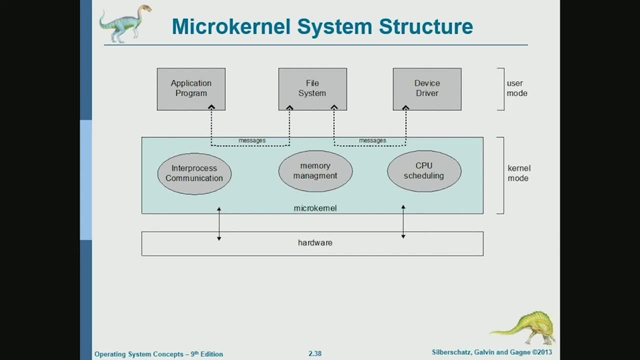 It's always more secure to minimize the code that is running in privileged mode. So the code that is running in privileged mode or kernel mode here is minimal And there is a security advantage. Yeah, You can swap out. you can upgrade parts like the file system and driver without having 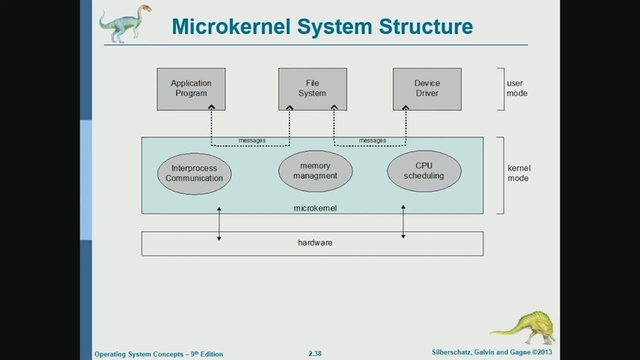 to update the kernel. Yeah, exactly, And updating the kernel here means recompiling the kernel. Remember that the kernel is written in a high-level language And if you know, the designers of the system, the developers of the system, the developers. 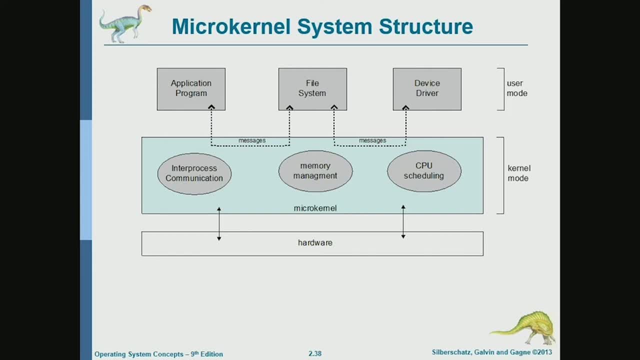 make a change to this service. they only need to recompile this And they don't have to touch the kernel. So they don't need to recompile the kernel. Okay, So this is a big advantage. You know, the kernel is small and it has only the essential features. 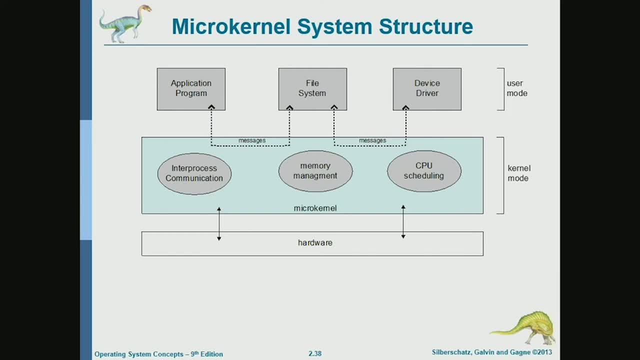 So recompiling the kernel will happen less frequently. Okay, Other advantages: If the driver system or application program is compromised in some way, we still have a somewhat functioning system as opposed to Yeah. Yeah, I guess if inside the kernel. 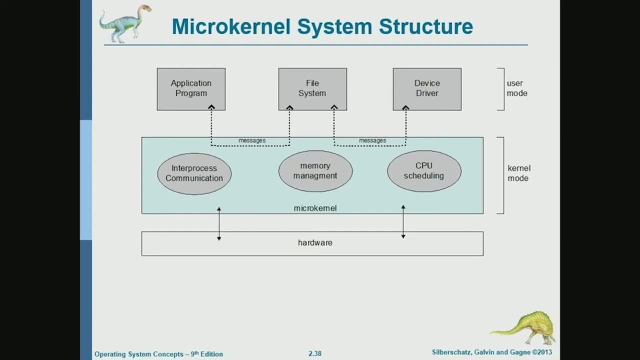 Yeah, exactly. So the question is what will happen if one of these services fails? If this service fails, it's not going to crash the machine because the kernel is still intact. Okay, So if one service fails, the kernel will not be affected and the system will still be stable and running. 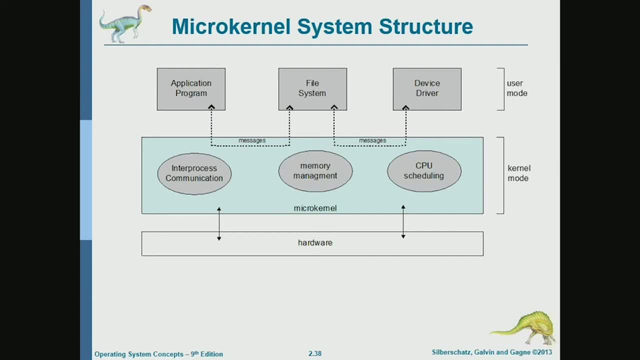 Okay, Yeah, So smaller kernel is, you know, more stability, because if anything goes wrong in any of these services, something goes wrong in any of these services, then the system, the whole system, will not crash. Okay, And there is a portability advantage. 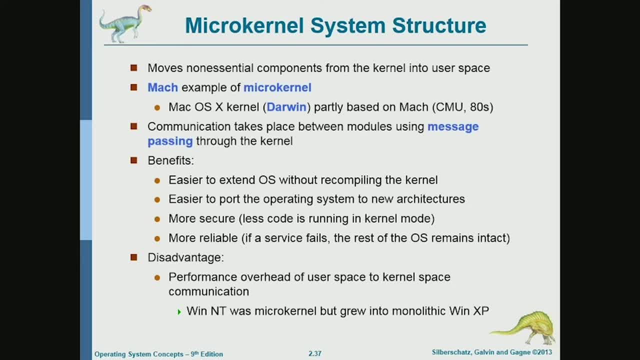 So when you have the system divided into smaller pieces, it's more manageable and it will be easier to port to another platform, because you- only you- know there are parts that are platform-dependent and parts that are platform-independent, And only those parts that are platform-dependent need to be ported to another platform. 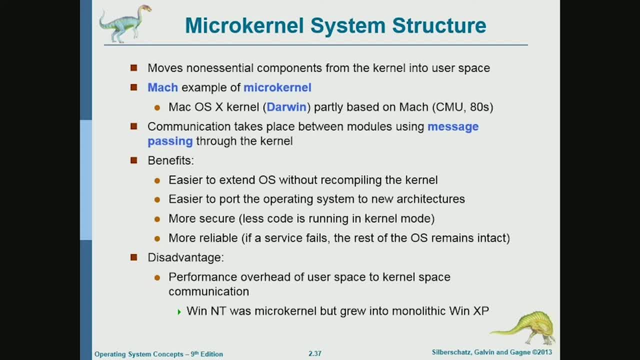 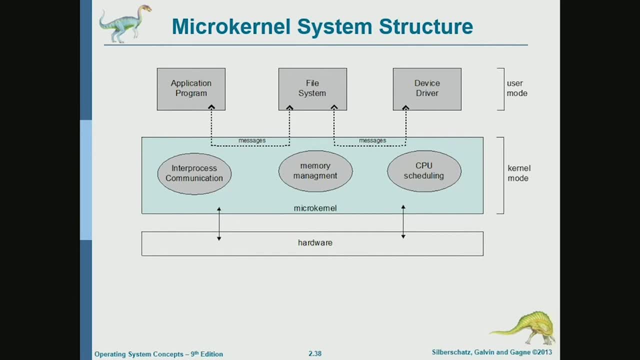 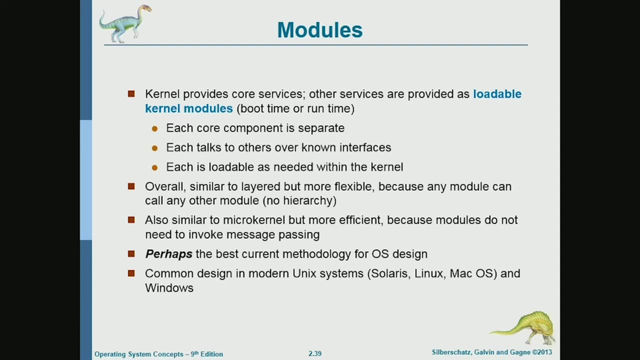 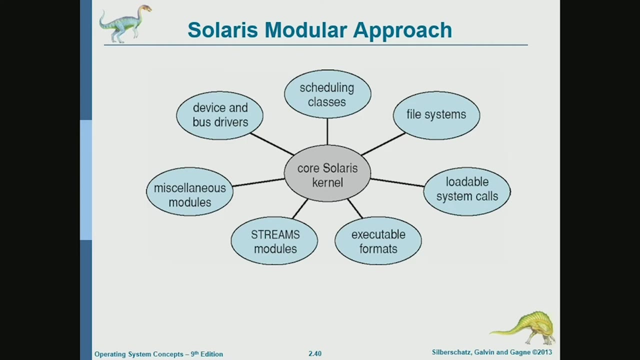 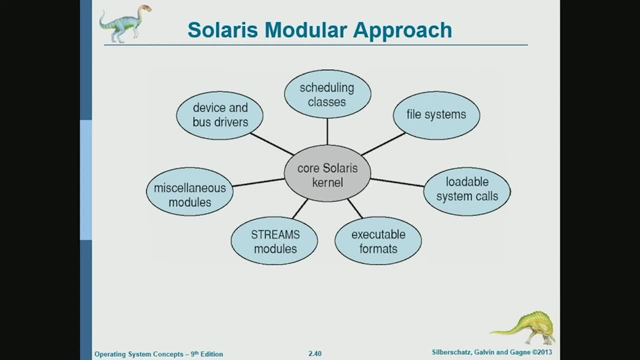 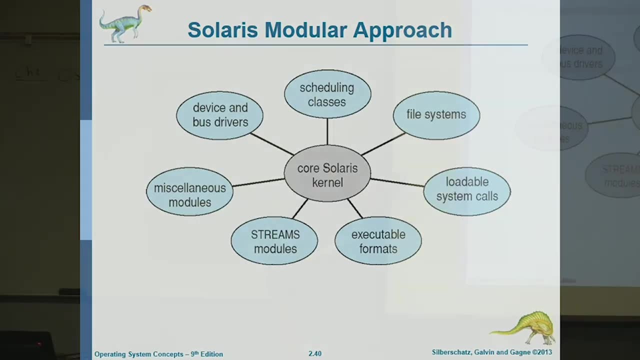 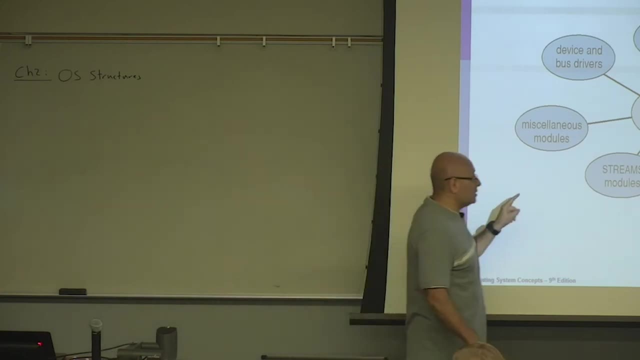 In the loadable module. it's very similar to the microkernel. So there is a similarity in the sense that there is a small kernel that has the essential features and all other services now are in modules. Other services are in modules that are loaded by the kernel. 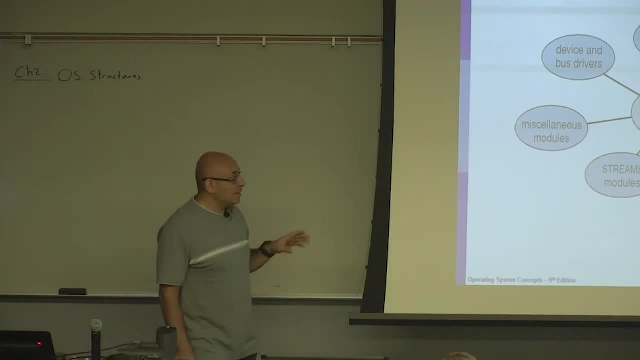 But the difference is these services that are not in the kernel, they are not loaded as separate processes, They are loaded as modules that are added to the kernel, So they are loaded as dynamic link libraries, for example, And one way of loading services is loading them. 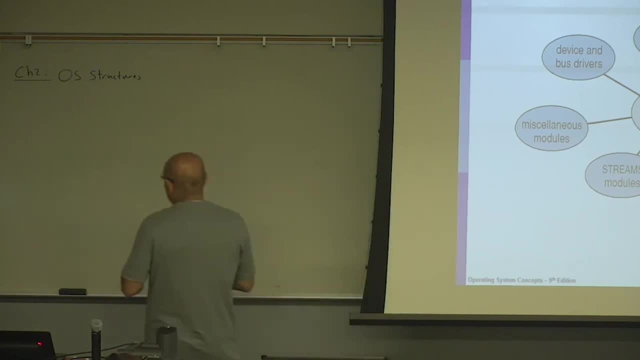 as dynamic link libraries and sticking them to the kernel. So in memory, the memory image look like this: So this is the microkernel. With the microkernel you will have your small kernel and then you will have the other processes as other services. 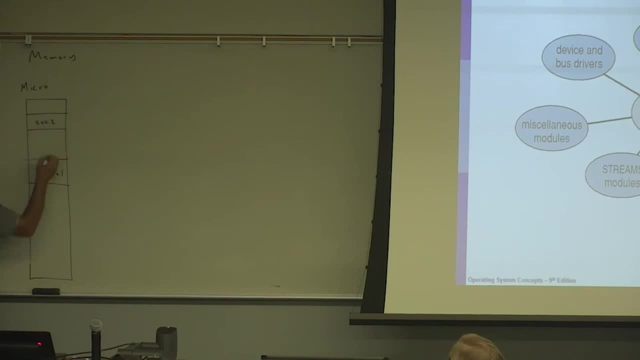 as separate processes. So you may have service number one, service number two and service number three, Three different services, And each one is a microkernel. Each one is a separate process and each one has its own address space. So this is the kernel address space. 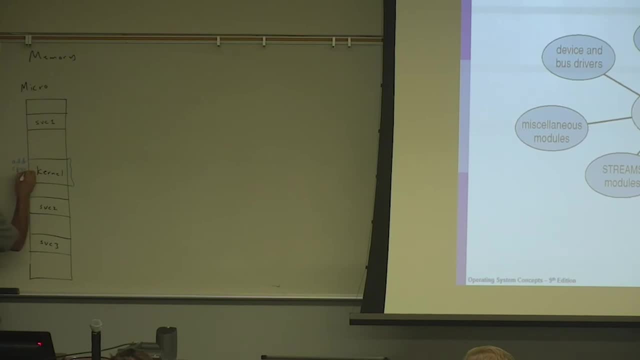 Address space. Other services have their own address space. Now with the loadable module, it will look like this. It will look like this: This is your small kernel, But then you load other services and you stick them to the kernel. So there are kernel extensions. 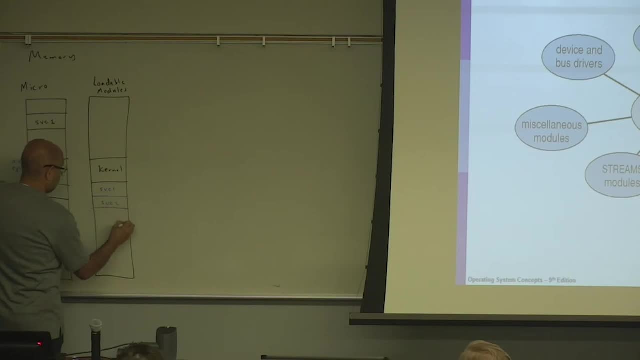 So I have service one, service two and service three, And this is one address space. So here I have one address space, Here I have multiple address spaces. So this is the difference between the laudable module and the micro. Now the monolithic is going to look like this: 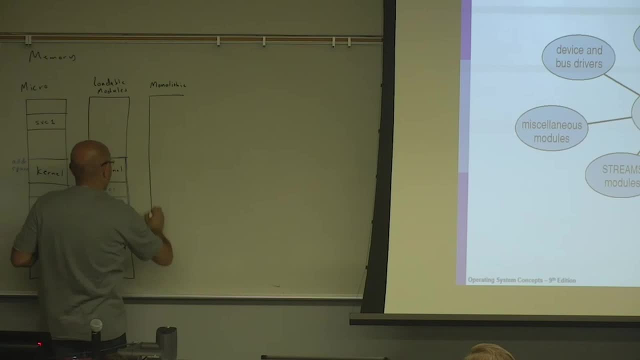 The monolithic is going to look like a big kernel. Now the question is: what will the layer look like in memory? In fact, layers will just look like monolithic in memory. Why? Because you're not loading new services into the memory. 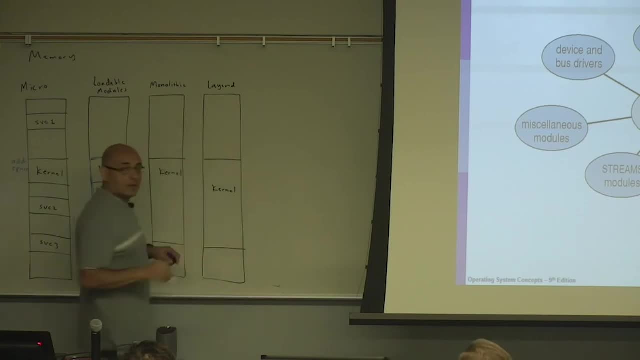 It's all there to start as layers there. Okay. So then what? where is the difference between layers and monolithic? Well, the difference is not in the memory image, So in memory, monolithic and layers are going to look the same. 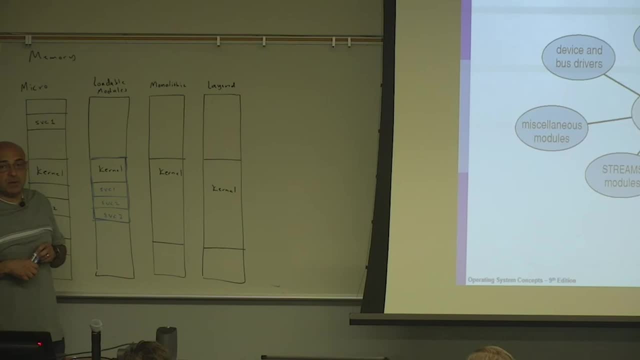 The difference is where. It's not in the memory, It's in the source code. So there's a difference. you know, if you look at the source code for monolithic and source code for layer, they will look different because layers will have a different layer. 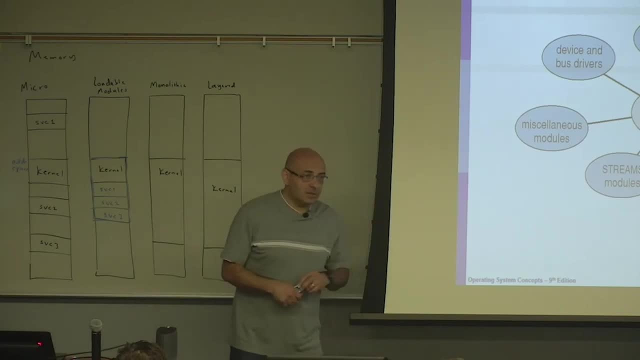 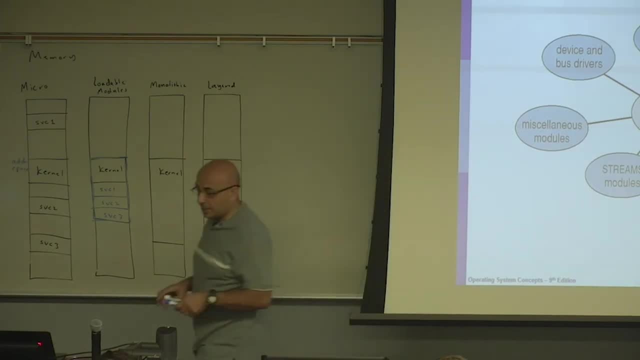 we have the hierarchy, But once that gets compiled into an executable or a binary, that binary is going to be a big binary like the monolith. So in the binary you will not see the difference. Okay, So these are these different approaches. 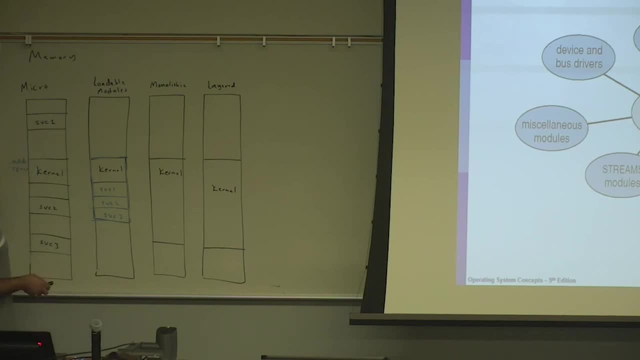 Okay, so Now let's identify some of the advantages of the module- loadable module- compared to layered and microcontroller. So what's the advantage of loadable modules relative to microcontroller? Your services are in continuous address spaces, so I guess there's less overhead as far as access time goes. 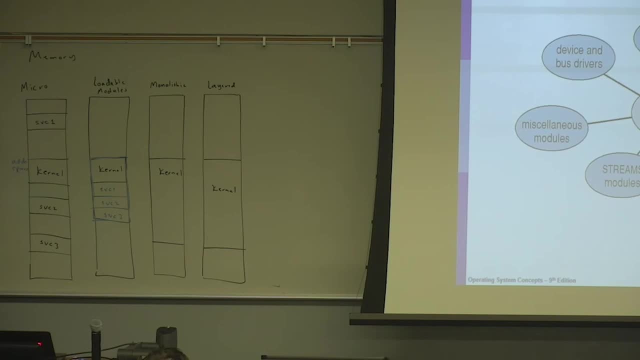 Well, what kind of overhead? So you know the word overhead is generic. It's not using your kernel and the services. So we, you know we talked about the overhead. We were very specific on the microcon, So there is something specific that we mentioned. 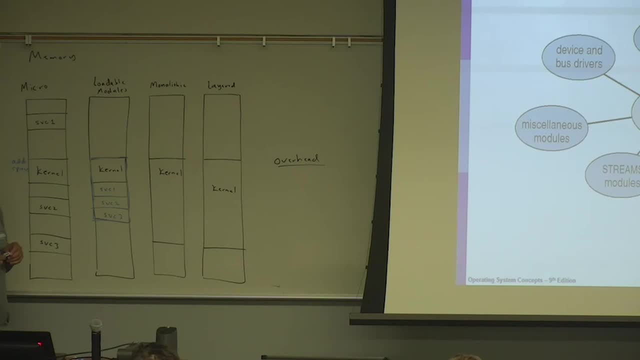 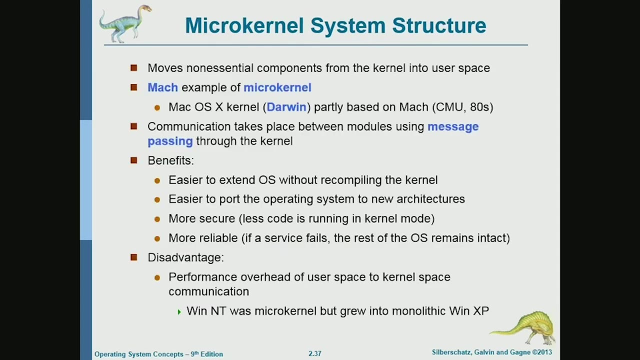 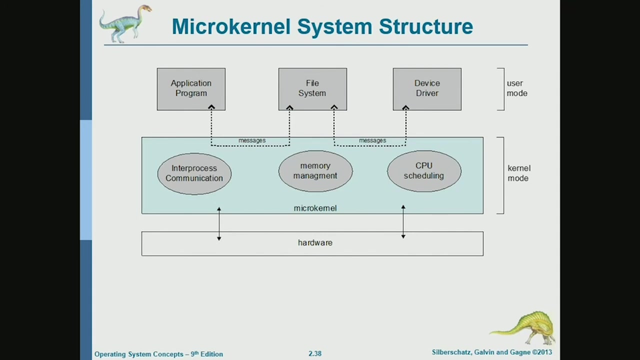 Like the process inside the kernel, don't have to go through the kernel to get outside to talk to other modules or services. And how was that communication happening? So if we go back to the- yeah, so that's a specific answer. So we have messages in the microcon that we do not have. 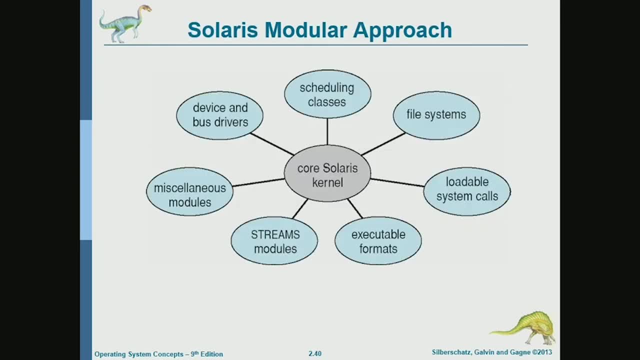 in the loadable module. Okay, So the question is: what's the advantage of loadable module relative to the layer? The layer, yes, It's more portable, so you can just plug and play the modules you'll need for whatever the device may be. 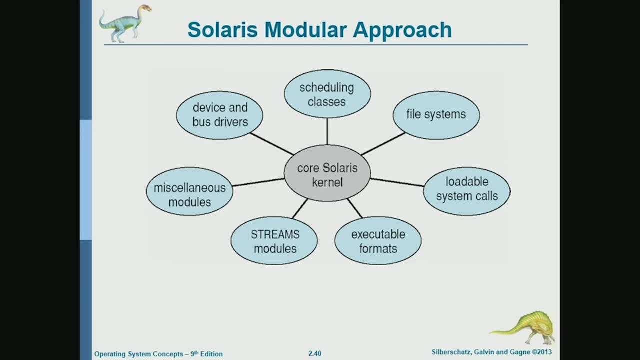 And you know you save memory space by not loading up some huge kernel. Okay, So memory is an advantage. yes, So memory is a clear advantage. Good, And I don't think of another advantage For loadable modules: do you have to recompile the kernel? 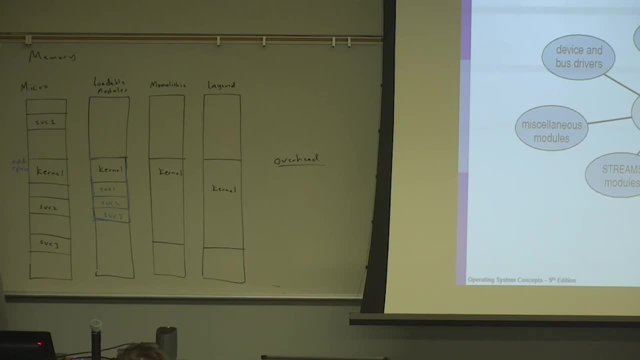 if you change one of the modules. Oh, do you have to? No, So these are loadable modules. They are loaded as modules, They are compiled separately, because when you compile, when you load them, you load them as libraries And you know you change service one. 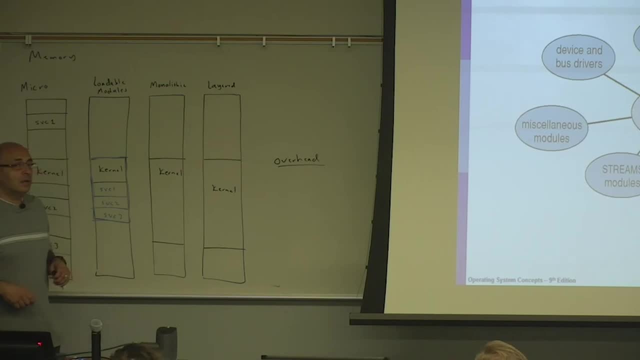 you don't have to recompile the kernel, So it's easy to update. Yes, Okay, That's true, So that's an advantage. Yeah, that's a clear advantage. Another advantage About the debug: yeah, but this is well-structured. 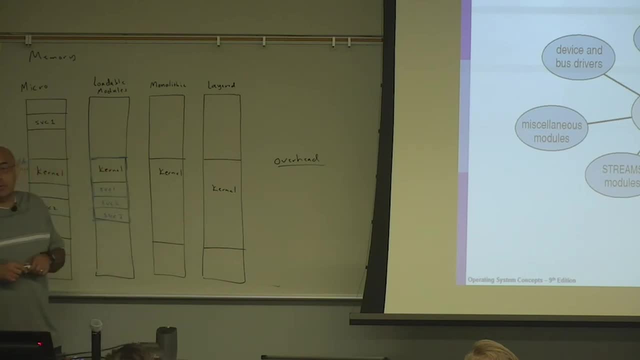 So debug-ability, this is good from debug-ability point of view. But what was the main disadvantage here in the layered approach? Better performance for the modular, Which has better performance, The modular, The layered, has poor performance. And why? 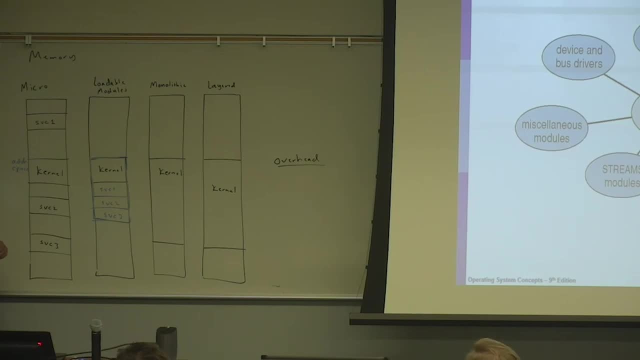 You can do work down through the all the through the layers, if you want to reach the bottom. As for the modular, one of you has talked to the module you want to talk to. Yeah, So, yeah, so here any module can talk. 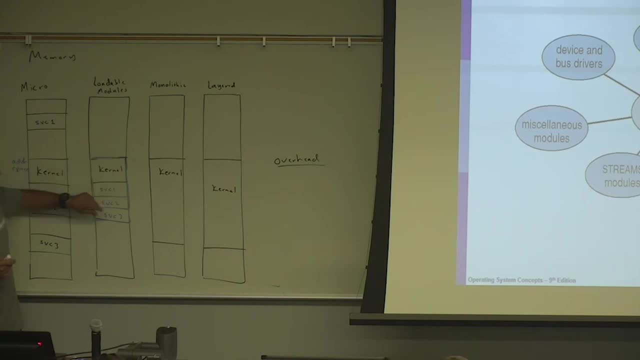 to any other module. So in the module any module can talk to any other module. You don't have to go through the hierarchy. But with the layers you are more restricted. So there's a restriction and you have to go top-down in the hierarchy. okay, 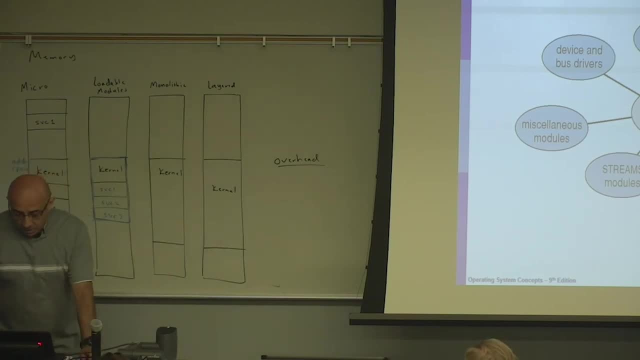 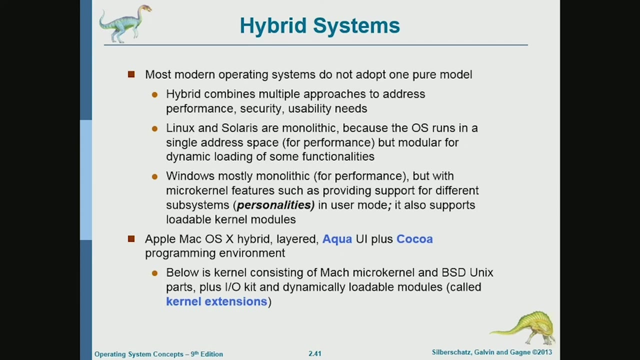 All right, so well. we have studied these four different kinds of structures and, as I said before, Noreal system implements one of these. you know, Noreal system implements only one structure or takes a single approach. All systems use. Noreal systems use a mix of approaches. 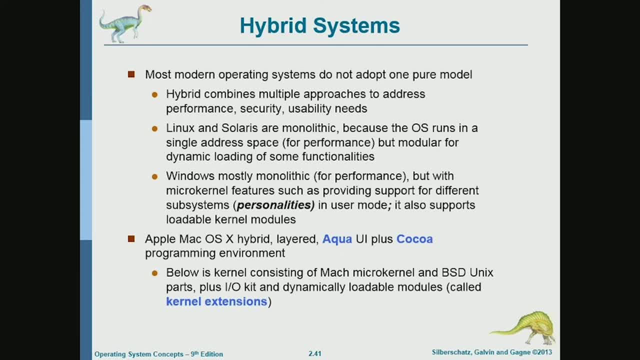 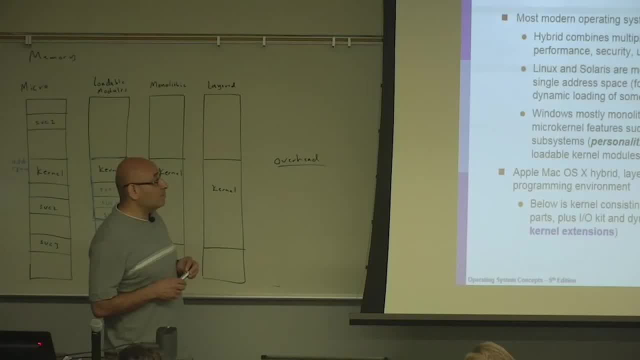 You know, for example, Linux and Solaris are monolithic to a great extent because the OS runs in a single address space. but there are modules, There are loadable modules. By the way, loadable, the loadable module approach is: 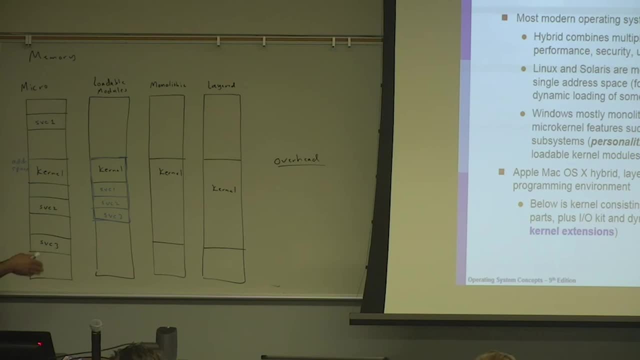 probably now. you know, in modern systems, I don't think it's going to work. It's probably the best approach, but it's not a perfect approach. So it's if you think about the advantages and disadvantages relative to other approaches, it has lots. 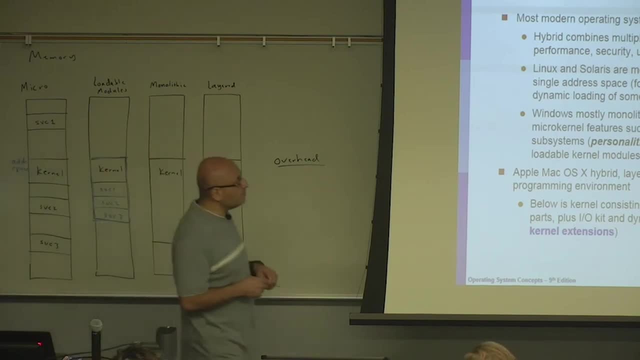 of advantages compared to other approaches. Windows is a good example. Windows started as a microkernel, because Windows, you know, is a microkernel. Windows NT was based on the VATS operating system, which was a microkernel. Then they realized that they have a performance problem. 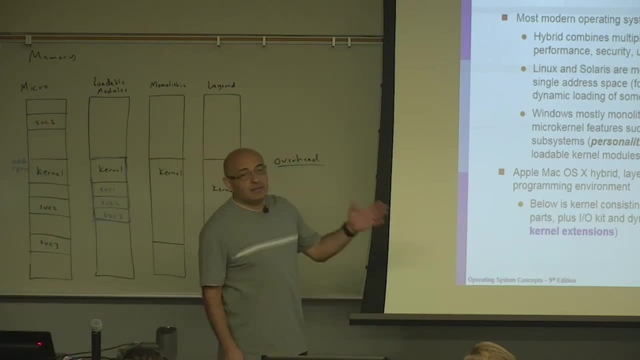 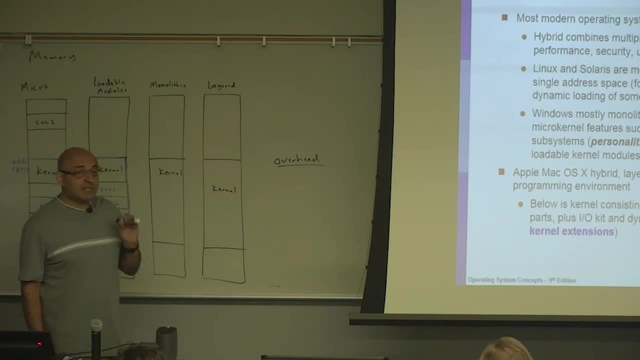 Windows NT, Windows NT, Windows NT, VATS, Windows NT. Windows NT is more monolithic because it's big, but still it's not a pure monolithic kernel because it still has some of the microkernel features that they were in the earlier versions. 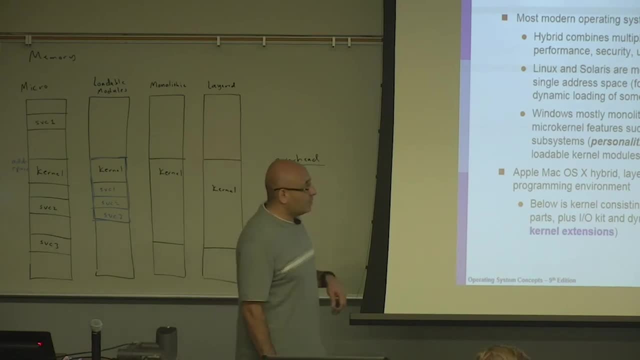 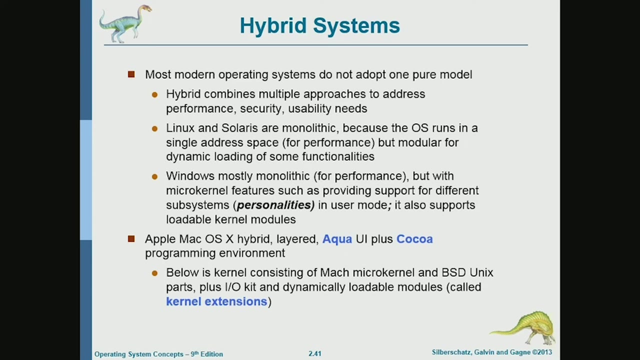 And it even supports loadable modules, Or they call, you know, sometimes called subsystems or personalities. So the subsystems are microkernel features, But there are also loadable modules that can be loaded. So you have a mix of micro-kernel loadable. 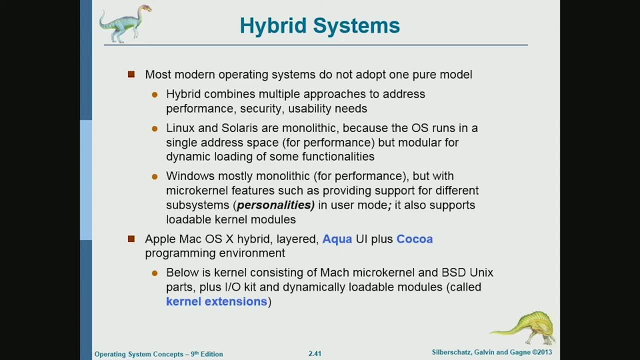 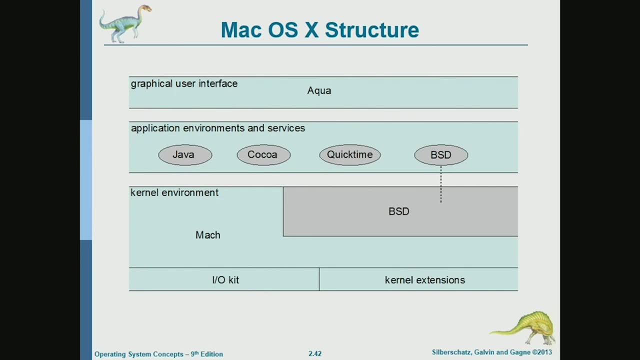 and monolithic because the kernel is very big. It's relatively big, Okay, And of course it's big for performance. The Apple Mac OS. so the Mac OS is based on the Mac operating system that was developed at Carnegie Mellon in the 80s, but the you know. 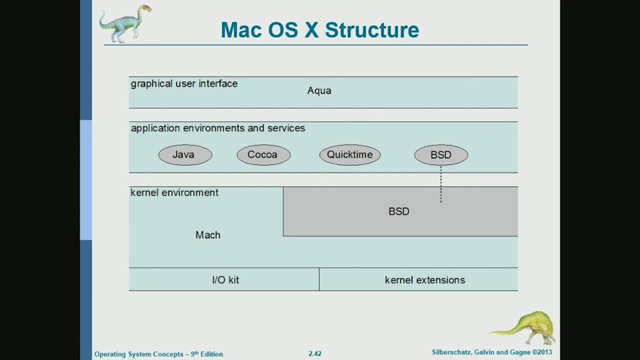 this is the Mac. the Apple's Mac with C and no H. that the Mac with CH is the system that was developed at Carnegie Mellon, But Apple's Mac is not. Apple's current Mac is not based totally on the Mac OS. There is also the BSD units as well, so it's a mix of two systems. 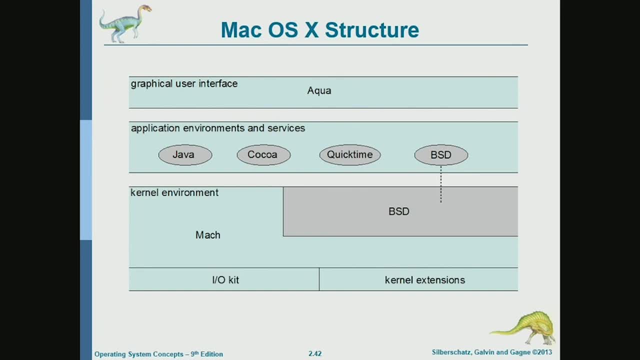 So it's all obviously a hybrid system and the kernel has a. it was based on two different systems and this- and it's a big, a relatively big kernel, So it's to a great extent, it's monolithic. 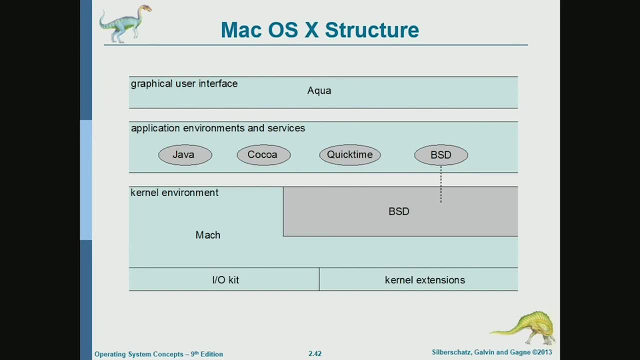 but it also supports kernel extensions and these are loadable modules, So it's monolithic, So it has loadable modules in it. So so far all the systems that we have looked at have loadable modules. All the you know system, Windows, Linux, Solaris. 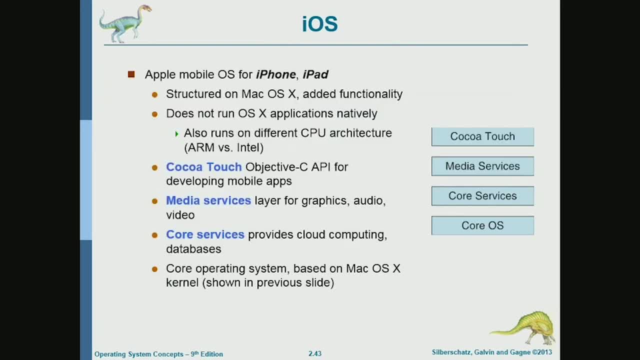 they all have loadable modules. The iOS, Apple's operating system for mobile devices- iPhone and iPad. it's similar. It's based on their Mac OS, so it's the core OS is the same as their OS for for laptops. okay. 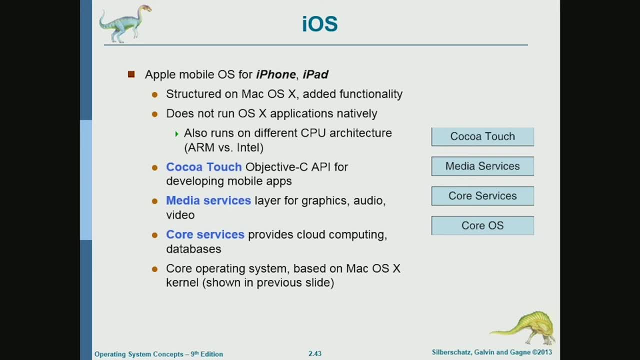 But it's. they added some layers that to support the mobile environment, including, you know, core services like cloud computing and databases, media services. So, as you can see on the screen, like you know, graphics, audio video and the Cocoa Touch. 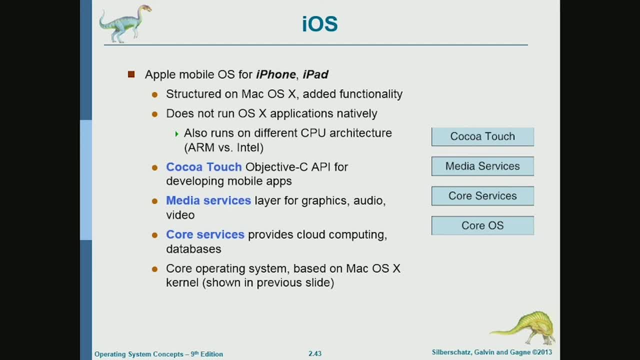 which is the user interface for the Apple in the Apple mobile devices. So it's it's based on the on the Mac OS, but you know it's so they're run on different CPUs. So you know you can see on the screen. 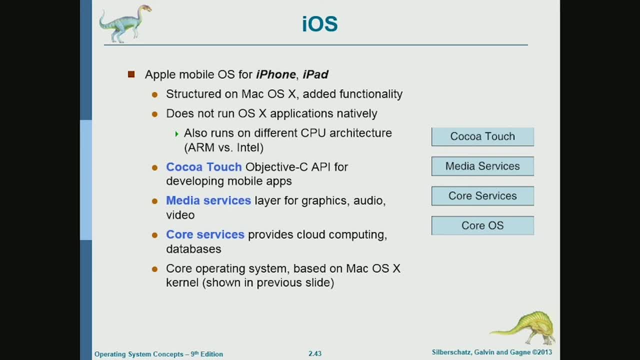 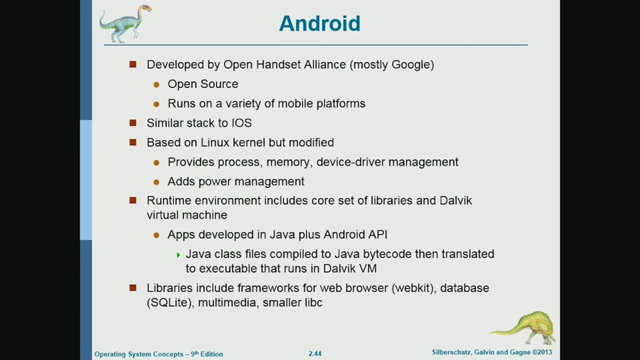 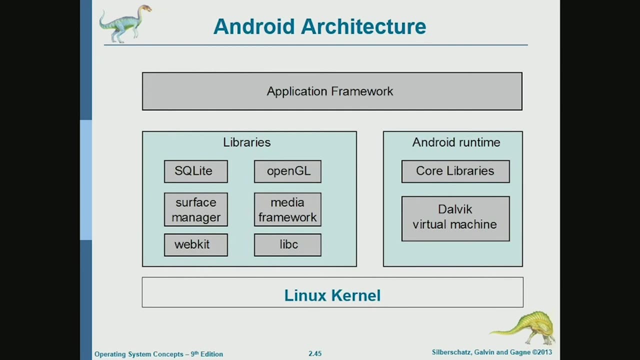 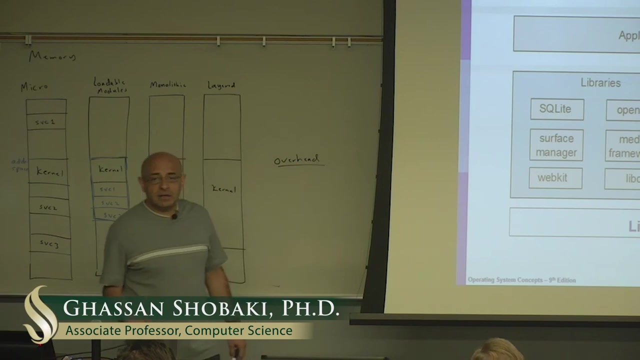 The Mac OS is run on Intel, while the mobile uses ARM processors. And finally, let's talk about Android. So the Android OS is based on a Linux kernel, And on top of that they added libraries and runtime systems to support the mobile environment. 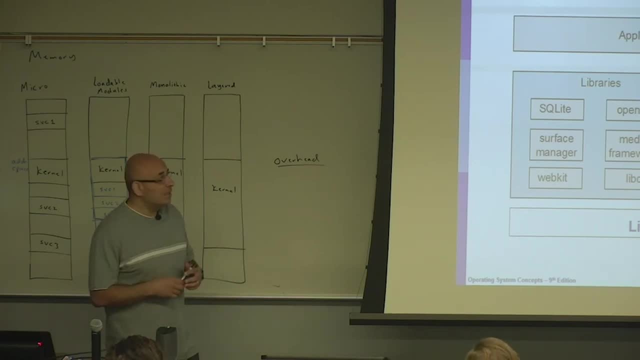 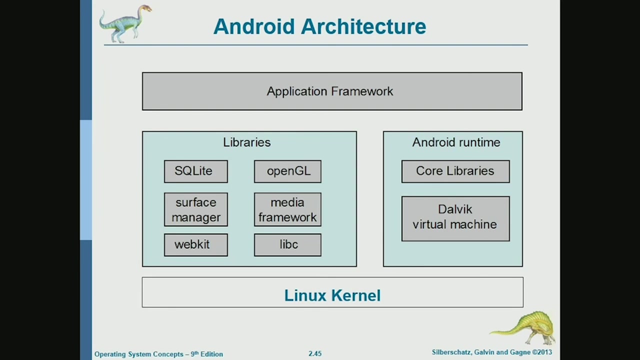 So it's Linux kernel plus additional libraries and services to support the mobile environment. Among these libraries we see the SQLite, a lightweight version of the SQL database. Lipsy- again it's a lightweight version of the C library, And the Android runtime system is based.